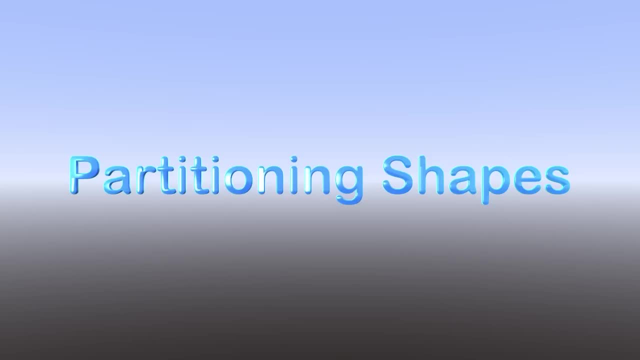 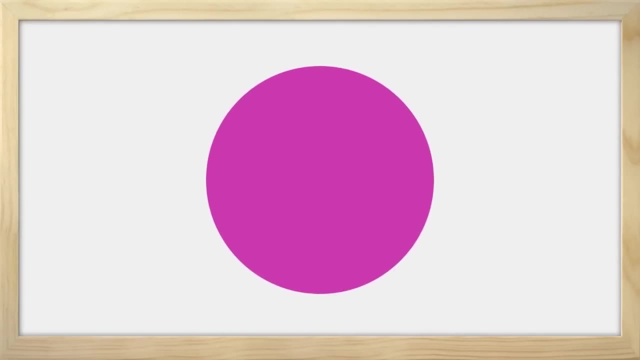 This is why we are learning about fractions today, so I can know how to make it fair for everyone. Here is a circle and there are three of us who want to share the circle, so I broke off two pieces and gave them to my friends. 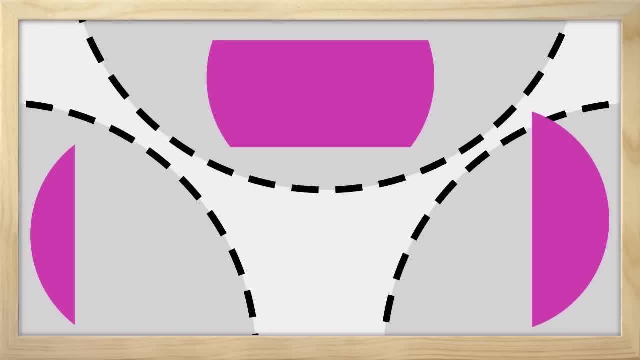 They did not think that was fair. What do you think? Do we each have even pieces of the circle? We do not, and that is something important about fractions: To be a fraction, you have to have equal pieces. Right now, we do not have equal pieces, so this cannot be a fraction. 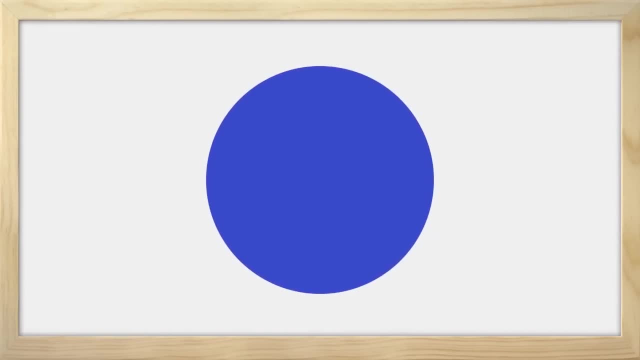 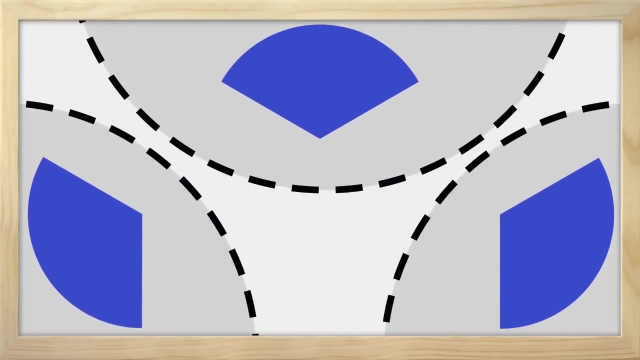 Let's try this again with another circle. Alright, here we have another circle and I am going to divide this whole circle into three pieces. Now we have three pieces and guess what? All equal, which means all three of us get the same amount of the circle. 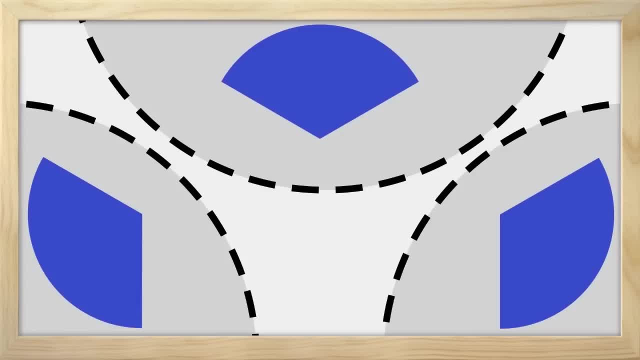 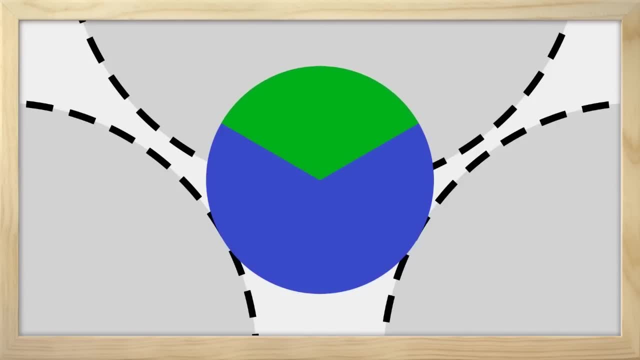 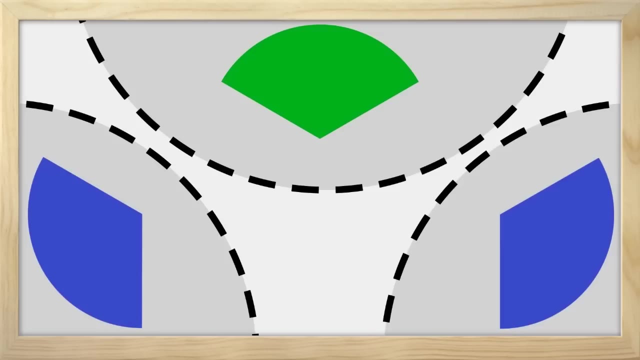 This is really cool stuff. I did not know I liked fractions this much. A fraction represents a part of a whole. The green part of the circle is mine to play with. I have one of three parts of the circle. We call this a third. 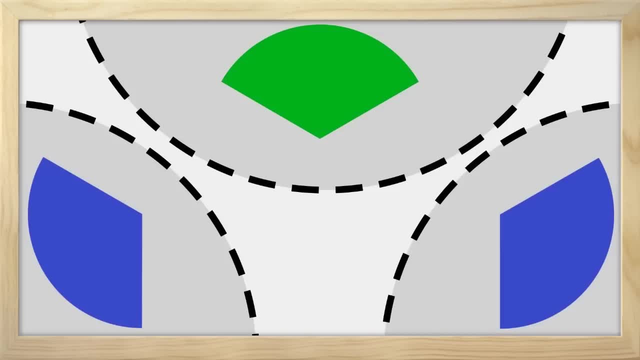 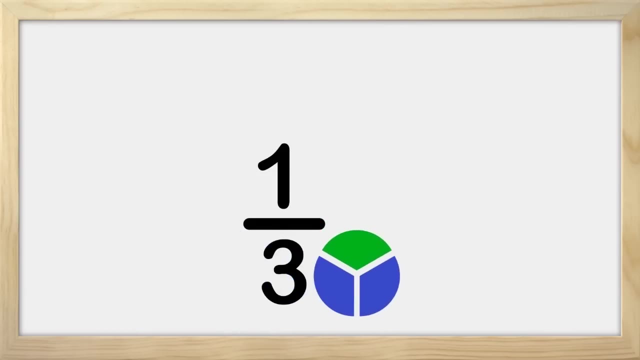 I have one third of the whole circle. When we write fractions we do not have equal pieces. When we write fractions they look like this: We have a number with a line in the middle and another number underneath. The number on the bottom always shows all the parts of the whole circle. 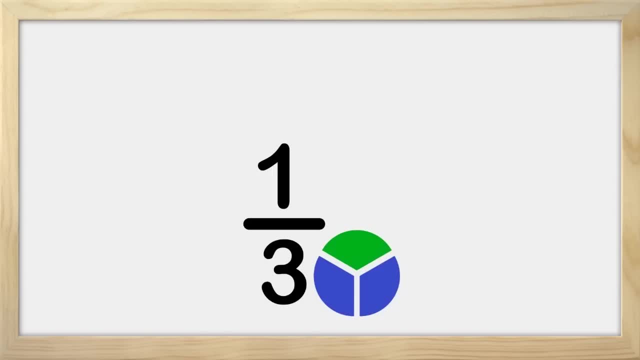 In this case we have three parts that make up the whole circle, so we have a three on the bottom. Now on the top we have the number one. If you look at the third of the circle that is colored green, you will see that there is just one part. 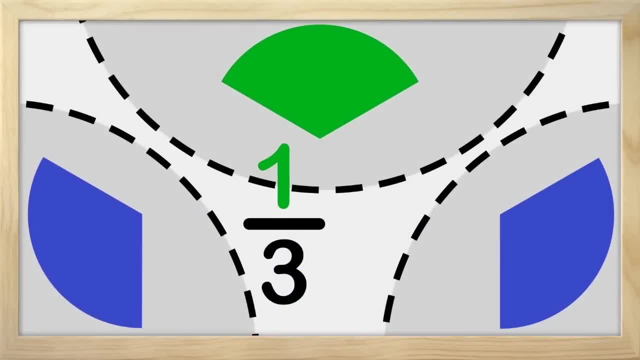 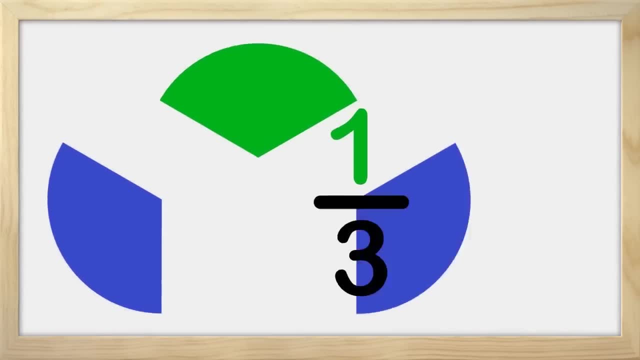 This is my part of the circle. The number one on top represents the third of the circle. The number two on the bottom represents my part of the circle. I have one third of the whole circle. Okay, my friends went home and gave me back their parts of the circle. 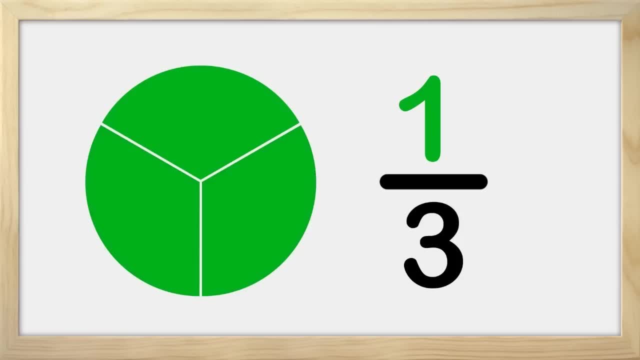 Now I have all the parts of the circle. I have what we call three thirds of the circle. I have three parts over the total, which is three parts, which means I have three thirds. This also means I have the whole circle all to myself.